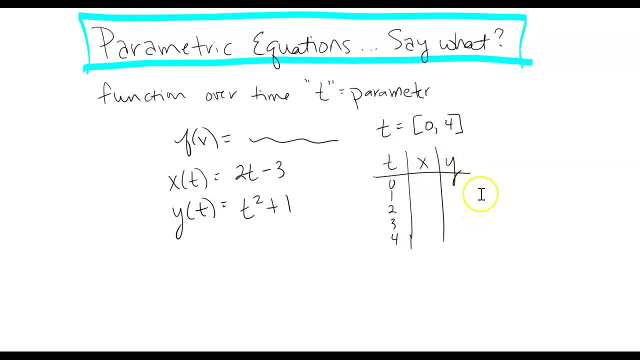 position at those different times. Well, how do you find your position? You just plug these fellas in to each equation, So it's pretty dang easy. So if I want zero, I'm going to plug a zero into both this one and this one and I'm going to get my position at zero. Let me make a little table out. 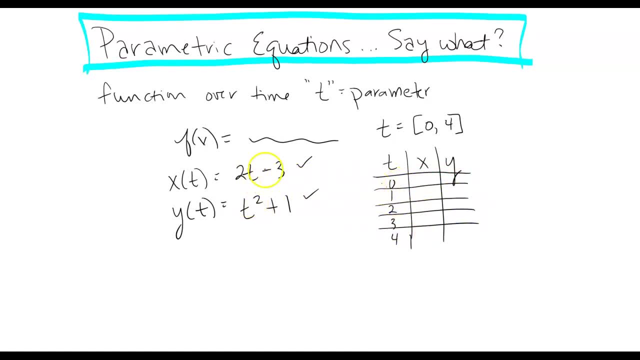 of this, All right. So if I plug in a zero to this- this is some quick mental math here- We're just going to get a negative three, And when I plug in a zero for the Y, I'm going to get a one. So that: 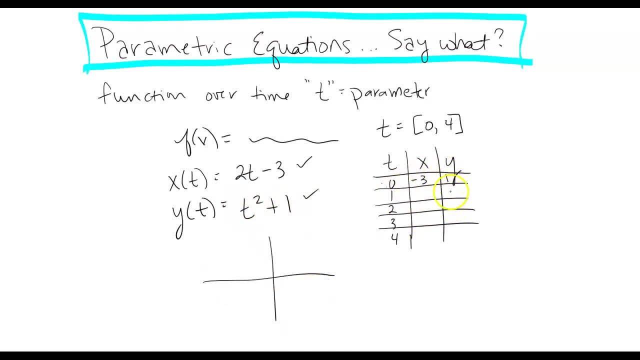 is my first position point. So when I go to graph it, I'm at negative three, positive one And that is going to be my point- when the time is zero. So notice, there's no axis for time, It's just happening in the background. This is still your X axis. This is still your Y axis. Okay, So now. 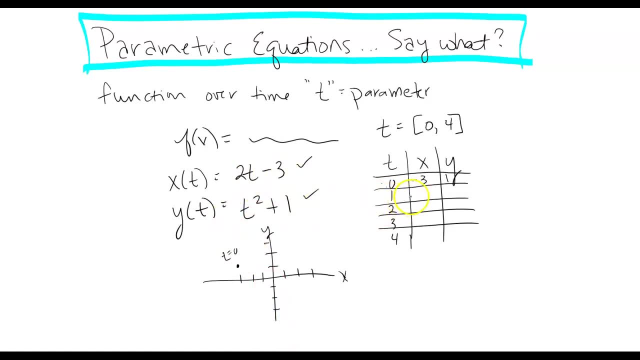 let's try one right. If I plug in a one, I'm going to get a negative three. And when I plug in a zero, two times one minus three is negative one. If I plug in a one there, I get a two. So at one second. 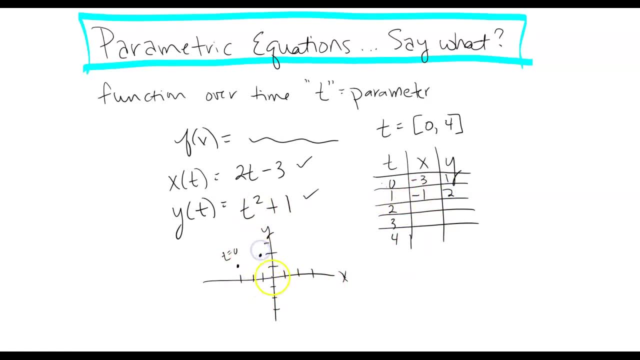 I'm at the position point: negative one, positive two. And then, if I plug in a two, I'm at the position one, five And notice there's starting to be a curve to this. So what I like to do is, when I sketch my parametric, I like to show direction, So I'm going to put little arrows. 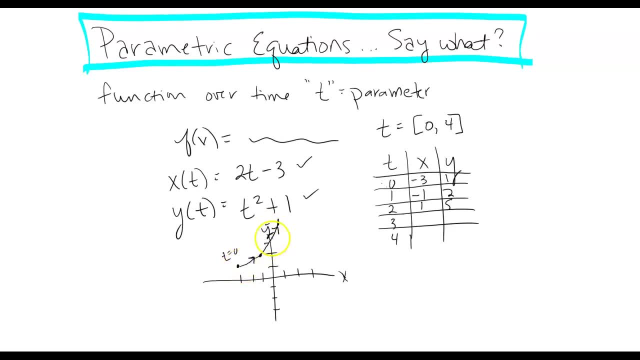 on this so that I know that, as time goes by, this is the way my graph is traveling. Now, when I plug in a three and a four, these data points are actually going to be way up here and I'm going to be out of room. So shame on me, um, for not thinking ahead, but you know what we can do to. 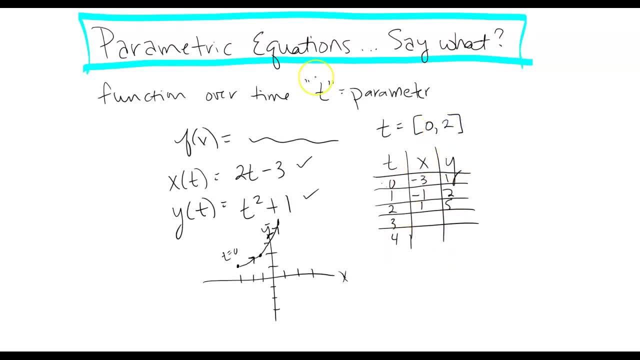 fix that. We're just going to change the problem. Let's pretend it just said zero to two, Voila, problem fixed, Okay, So I'm not even going to look at those. So basically, here is my curve. Now if you're wondering or if you're curious how that sort of makes sense in the world, 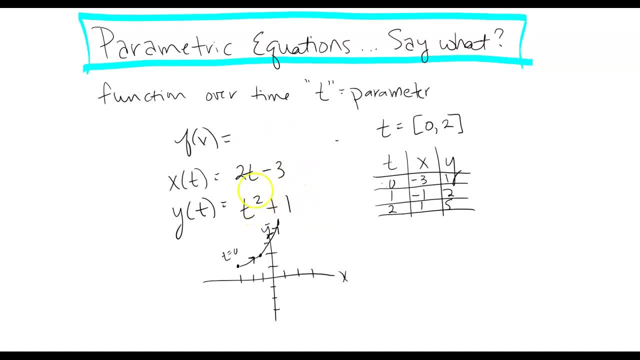 that we normally live in this, this function mode. there is definitely a way to go from X and Y back into function mode um or uh, what's called rectangular mode or Cartesian mode- All of those are synonymous. And the way that you do that is um, you eliminate the parameter. is is what people 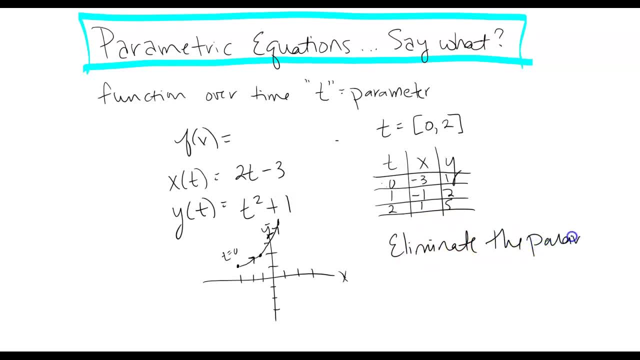 say in the math world, And if you're told to eliminate the parameter, it basically just means like get rid of T, get rid of time and go back to a normal F of X equation, And doing it is actually really easier than you probably think it's going to be. Um, all that we 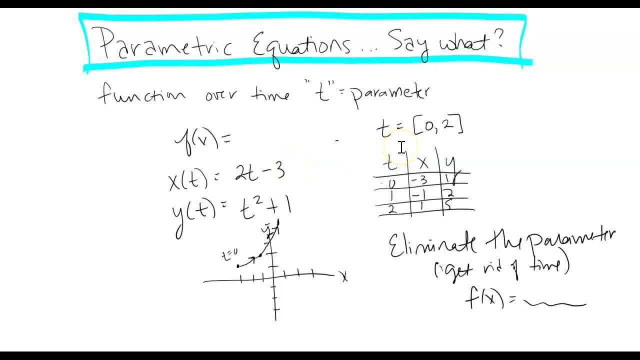 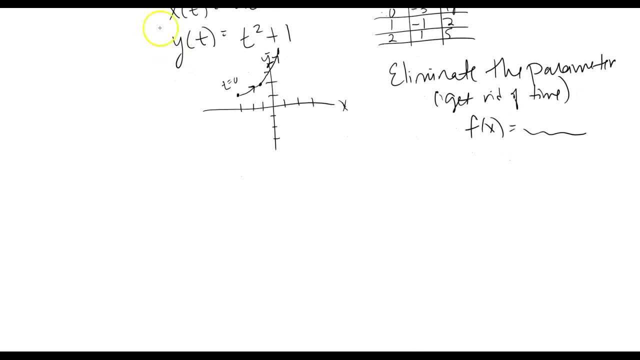 have to do is a little substitution problem. So, um, I'm going to scroll down, hopefully, so you can see. All right, So what's going to happen here is, um, I'm going to take these equations that I just have and I'm going to not think of them as functions, but just as a normal. 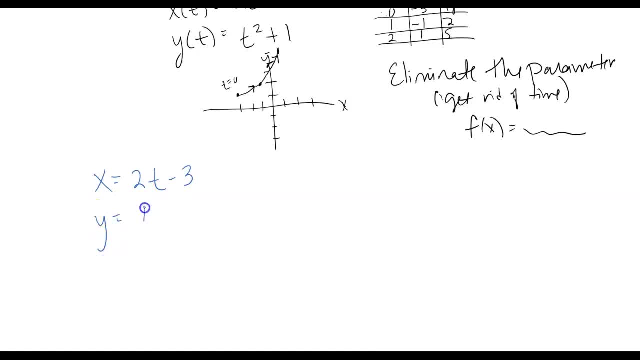 X equals two, T minus three and a normal Y equals T squared plus one, And my goal is to get rid of T and write it as an F of X equals or a Y equals. So what I like to do is I like to go to my X equation. 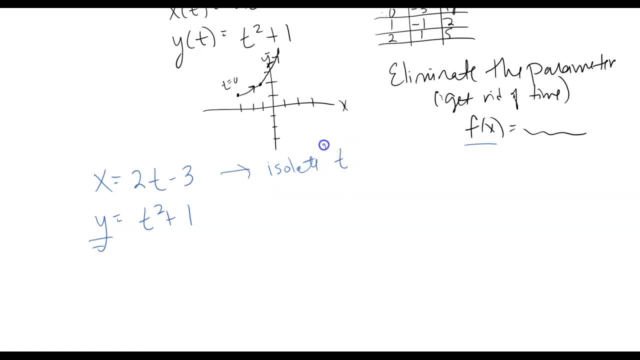 first, and I like to isolate the T, And after I do that, I then substitute it in to the other equation, and I'm done. So how do we isolate T? Well, on this one, we're going to add the um. 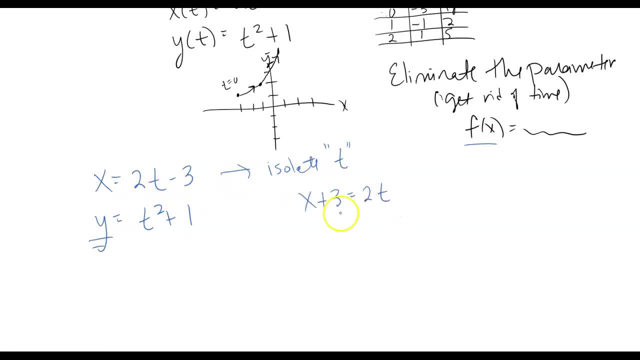 add the three to the other side, and then to get T by itself, we're just going to divide both sides by two, right, Okay? So T is now equal to X plus three over two. Now I go to my Y equation And: 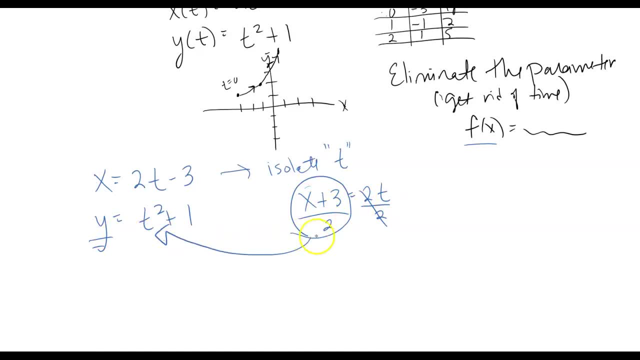 if T is equal to all that, then I can sub it in to its spot, do a little substitution, just like it was a system of equations or something, And this is my equation. So, really and truly, what you're seeing above is part of a parabola, right? And how do I know? 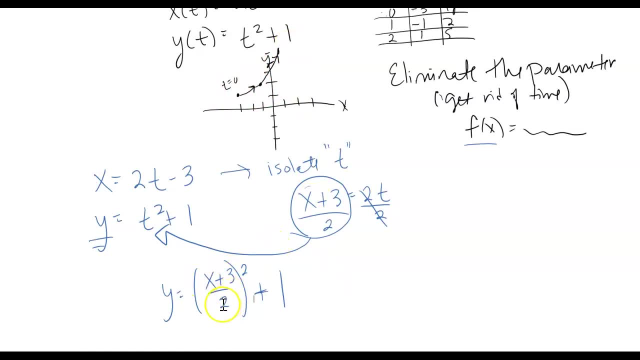 it's a parabola. Well, I have an X squared here, Um, this is, this is a parabolic term, So um, or equation, like a quadratic equation. So we're seeing part of a parabola and we could graph this. 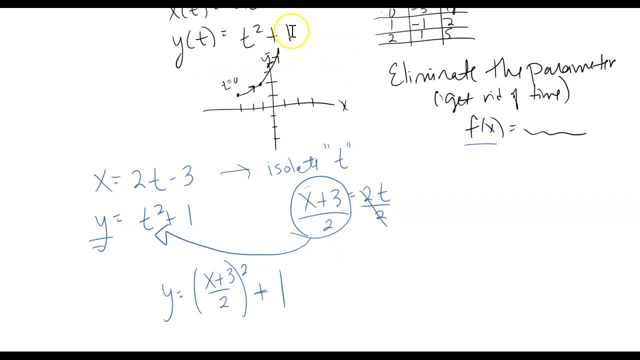 whole thing and guess what? It would in fact land on top of this? Um, it's just that we wouldn't see the time happening in the background. So that's kind of how this works. Now, why do I like parametric? Well, I think they're super useful to get to do cool stuff, For instance, conics baby. 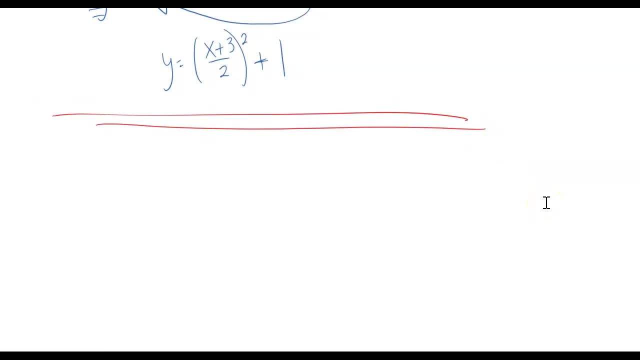 Uh, we just had a conics unit and we couldn't graph a dang thing on the calculator because well, uh, you just can't graph a function on a calculator, or so you thought, If you can take your conics and you can, 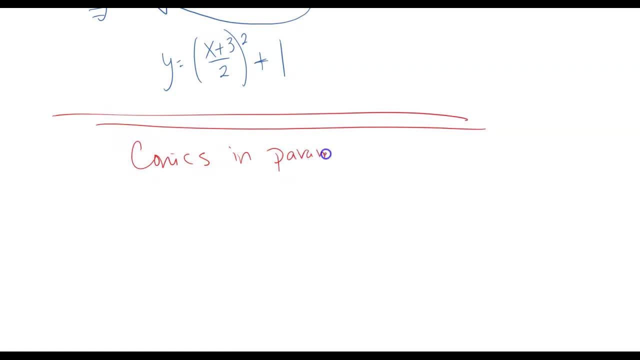 actually write them in parametric mode. you can, in fact, graph them in the calculator and check your answer and so on and so forth. And what I would ask you to do is is: I'm going to write it kind of a parrot function out so that you can take a look at it, but please do this in your calculator. 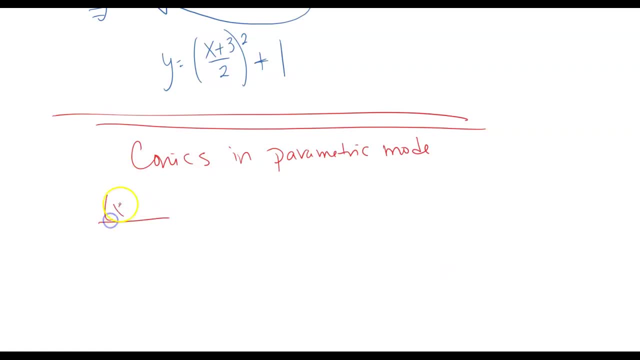 Um, let's take something in standard form like X plus one squared over nine, plus Y minus three squared over 16, equals one. So the first thing is: hopefully we all know this is the equation of an ellipse. Um, we know where the center is. The center is negative one three. We also know that. 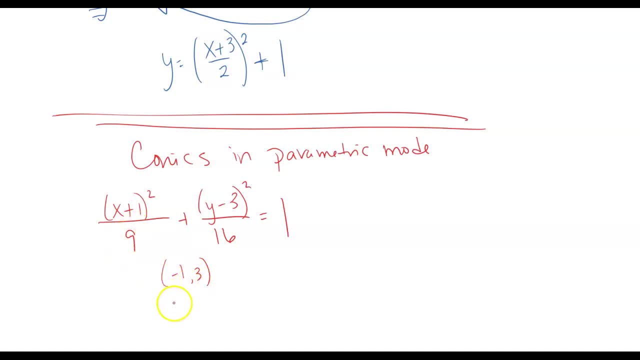 our radius for the X axis is really a three. Our radius for the Y axis is really a four, because we're taking the square root of those. All of that is stuff that you know how to do now in parametric mode. Okay, If you want your X and your Y equations. 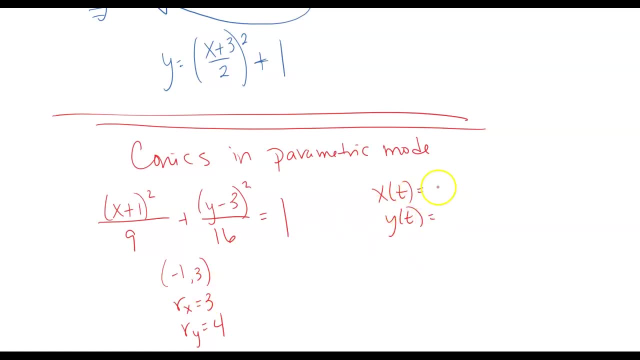 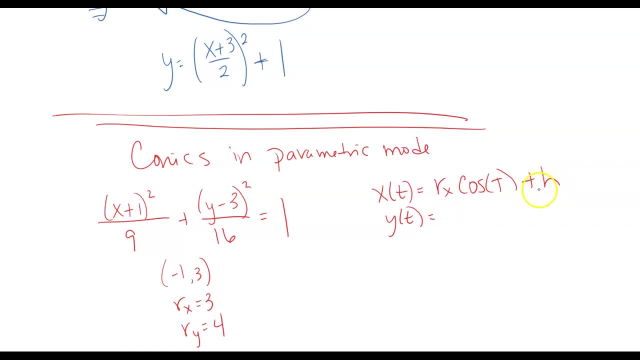 your plus H behind it. So if there was a shift um to the left or right, it's going to be very literal behind there And for your Y it's going to be the Y radius times, the cosine or sine, Just. 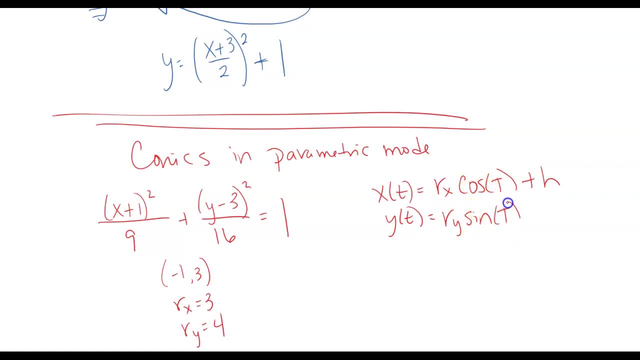 make sure you have one of each. Okay, It doesn't matter where they go, but you need to have one cosine and one sine, And then you've got your K. So in other words, um, I could take this ellipse that I already know- or I should already know, kind of, what it looks like If I want to see it on the 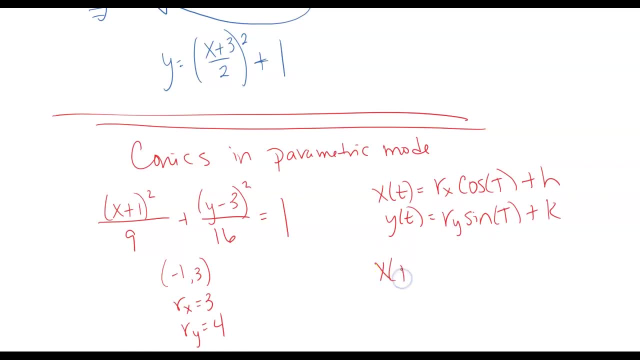 calculator. I'm just going to type everything in the right place And then I'm going to type it in there And it's going to be three cosine of T, And my H is really a negative one. right, Here's my HK, My center is my H and my K. These values over here are your H and K And my Y equation is going. 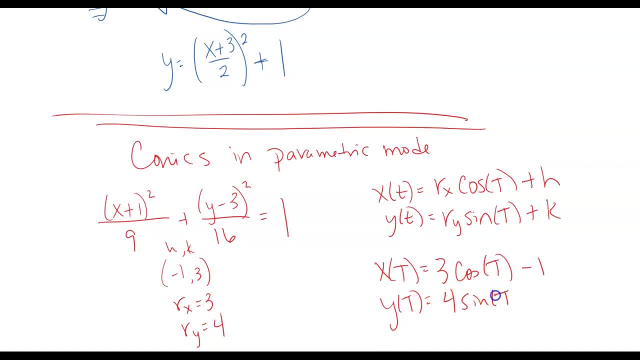 to be four sine T, And then what was my? was that a positive three plus three? So what I can do is go to my calculator, and I wish I had an online calculator To do this with you, but I don't cause, I'm not cool like that And I don't have money for that. 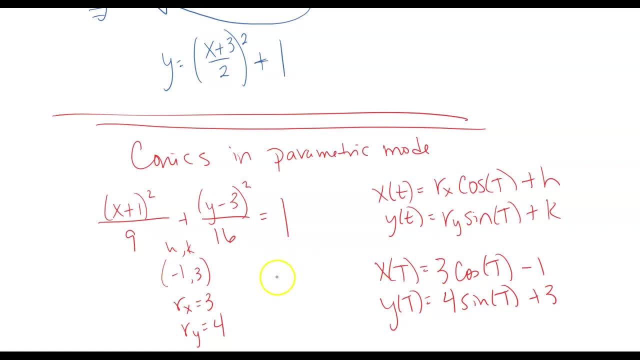 software. So shut up. Um, we're going to go to our calculator that's in our hands right now and we're going to hit mode. Then we're going to go to PAR mode for parametric and you're going to select that, So hit enter. Then you're going to go to Y equals and notice when you get to the Y. 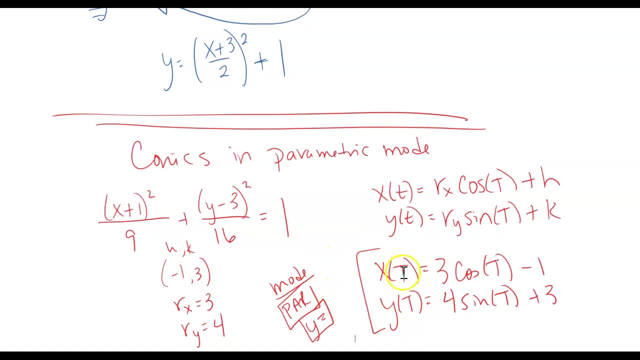 equals screen, y'all, you're going to see this. It's miraculous. And once you see this, you're just typing this stuff in. Now don't overdo it. You're going to see this. You're going to see this. 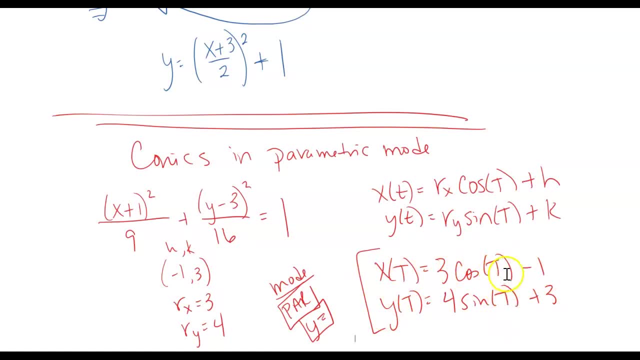 overthink the T. If you're like: where's the T? How do I type in the T? Okay, Guess what? That little button that you always use for X. look closely at that little button. It's got an X on. 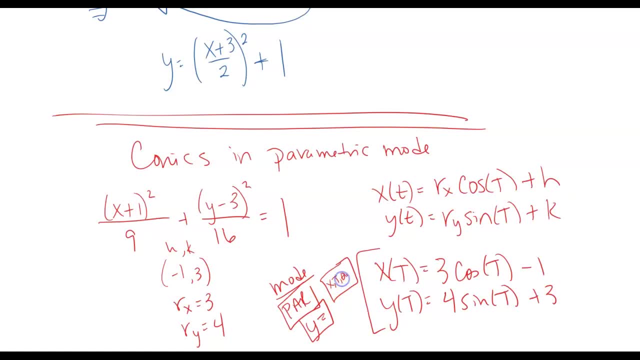 it. It's got a T on it, It's got a theta and it's got something else, an N. maybe If you hit that same button it automatically knows to turn it into a T for you, But anyways you could type. 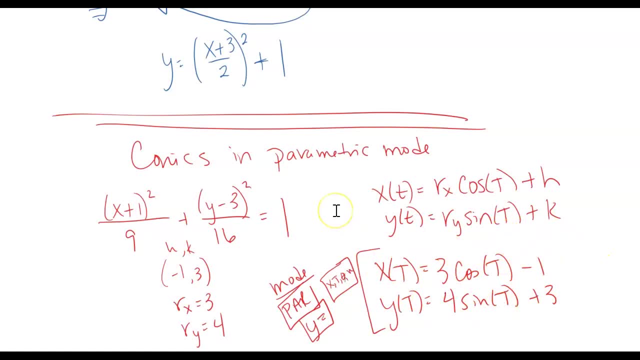 this all in. You can hit graph and guess what You're going to see: your cute, adorable little ellipse. Isn't that cool. So this works for both ellipses and circles, right? So the only difference on a circle is that these two numbers would be the same. Hopefully, we all know that. 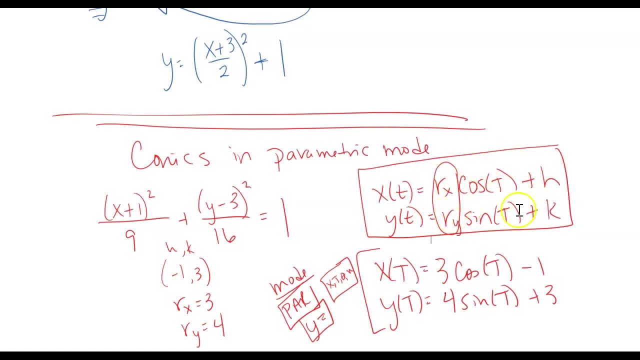 those would be the same if it was a circle, But it would work: the same, the same cosine sign. And then your center over here would be dictated by your H and your K. All right, cool. So how do I make a hyperbola? Because a hyperbola is a little different, right? Okay? So for a hyperbola. 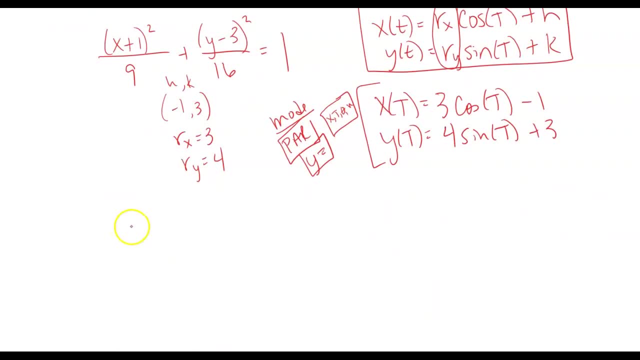 the parent function would work out sort of like this: Um, do, do, do, Okay, We still have our X and our Y, So this is a hyperbola, hyperbola, hyperbola, Okay. Um, on this one you don't use cosine and 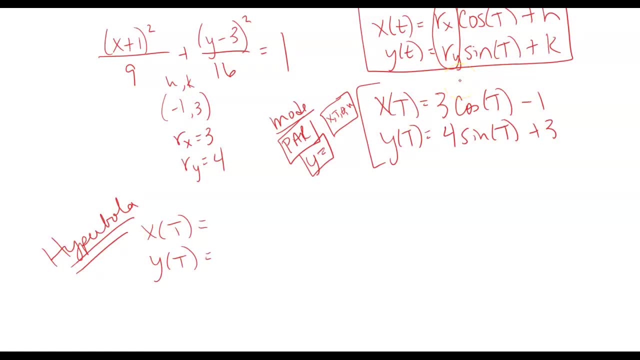 sine. You actually use two other, uh, two other trig functions. You're going to use your um, right, R, X, R, Y. You're going to use secant and tangent. And here's the kicker: where you put um, secant and tangent is going to dictate if it is a vertical ellipse or a horizontal ellipse. 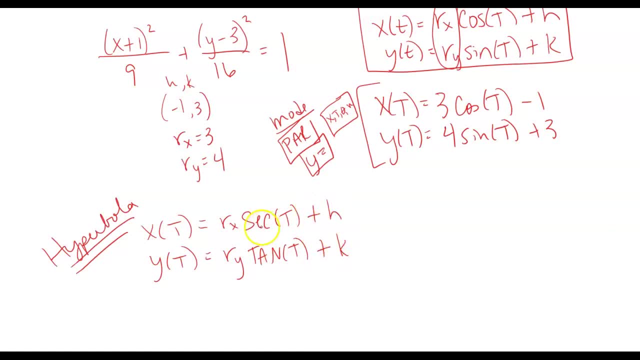 Now the way that I'm writing it right here, with secant going with X. this is going to be a side to side hyperbola. So if X is in the lead of your equation, remember if X is in the front, and then. 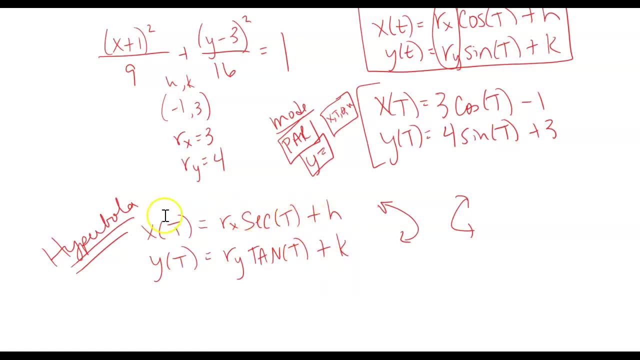 it's a minus and then a Y. you want the secant to go with X. If you were to flip flop those and you were to put your um tangent first, so it would be like R- X tangent T plus H and then the R Y secant T plus K. That's when you're 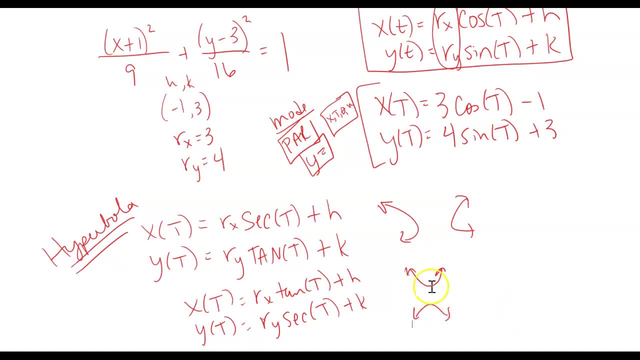 going to get an, a vertical, um, vertical hyperbola, um, because secant dictates the shape or the orientation. Okay, And that's pretty much how that works. Um, so feel free to try it, check it out And remember, if you're trying to type in secant, there is no secant button. 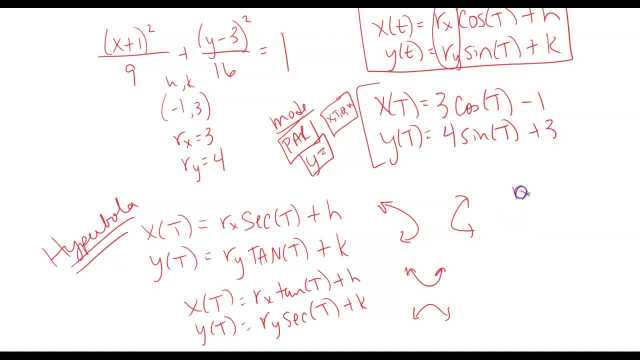 So you're going to actually have to type it in as sort of like your R X, um divided by the cosine, because, remember, a secant is equal to one over cosine. So when you're typing it in, there's a little tip for you. That's how you're going to have to type it in. 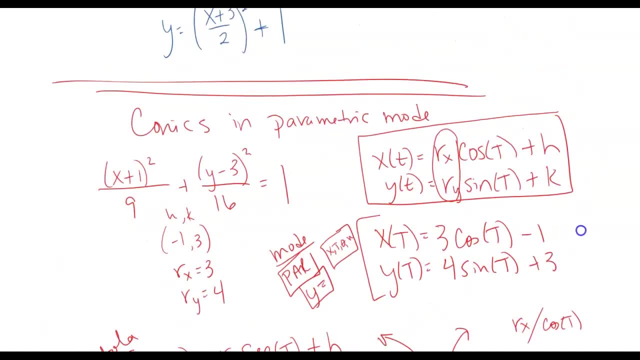 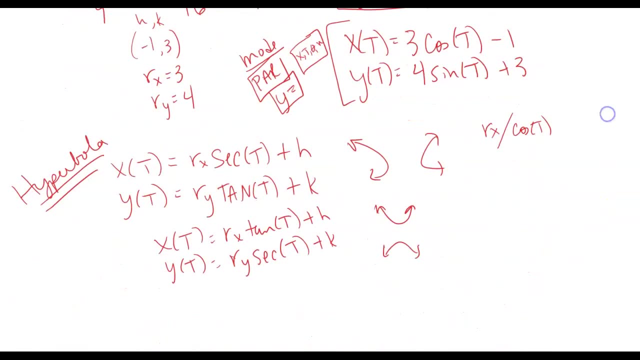 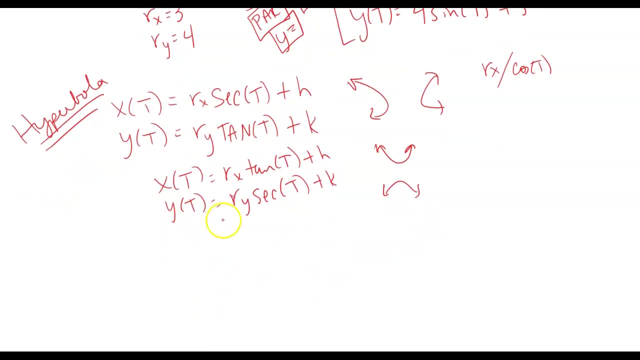 So that's how parametric works: Um, you can graph in parametric. you can eliminate the parameter. Um. you can also do your conics this way: Um, I'm not going to show you in the video, but you can also do parabolas. Um, and it's actually pretty basic. Uh, I want you to play. 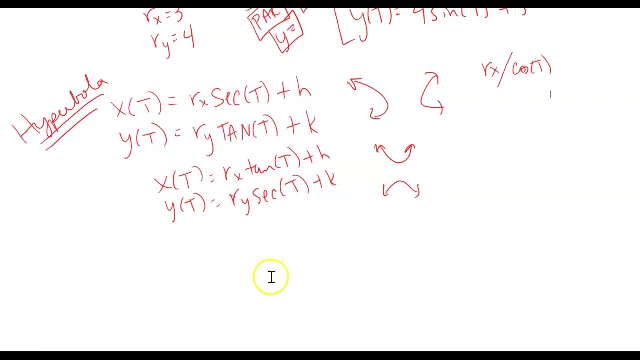 around with that and we can actually um do a little bit of a little bit of a little bit of a talk about that later. Um, next time I see you if you can't figure out how to do a parabola.